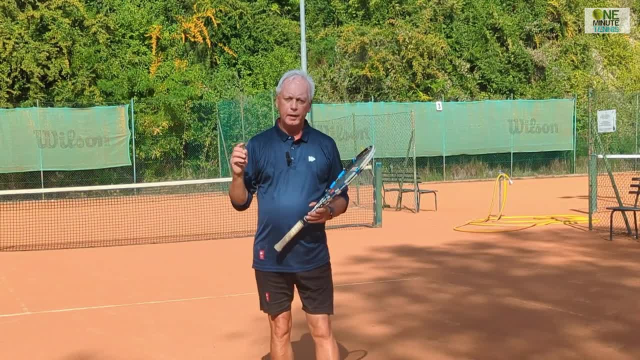 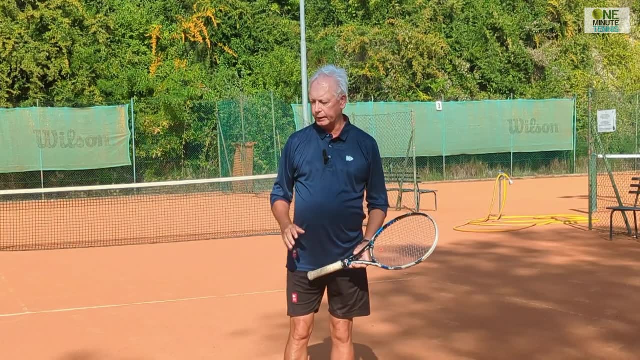 going to play this ball high, But that's not so difficult to do. And then, once you're aware of it, think about having a set of shelves by the side of you. So if I have a set of bookshelves here, then I have a low shelf and I have a medium shelf and I have a high shelf. So it's somewhere in the 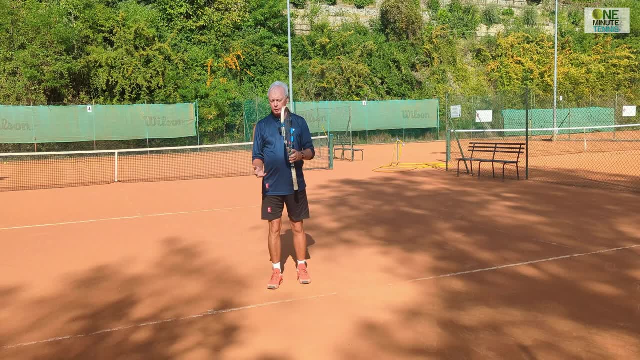 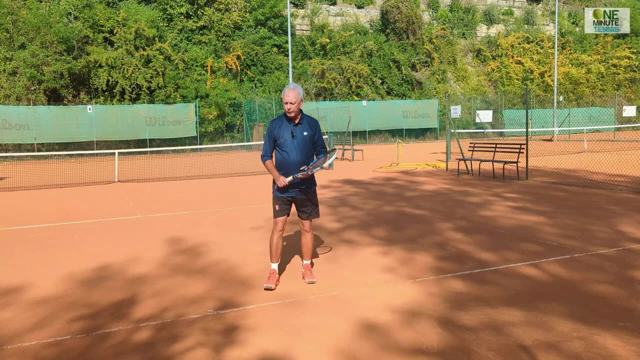 range of from here to down here, And the shelves are maybe maybe two foot six in depth, So maybe 60-70 centimeters for the depth here. So what I'm going to do is, if I get a low ball, then I'm going to set up around the top of that low shelf. 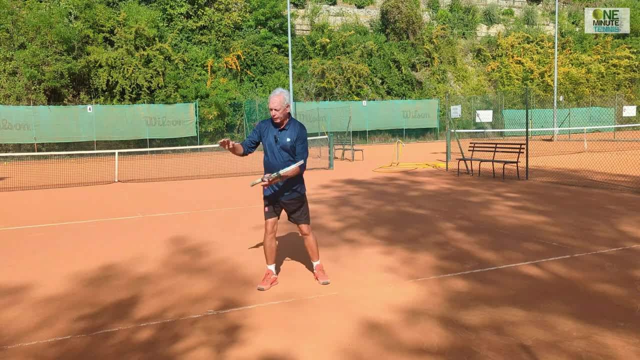 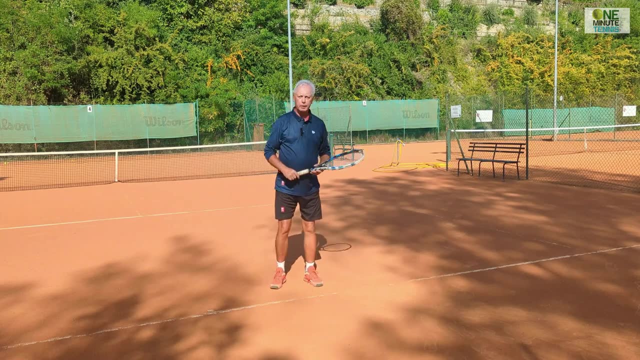 And then the racket will drop and I'll swing through. If I have a medium high ball, then I'm going to set up along the top of that shelf and then swing around the bottom of the shelf. And if I have a high ball, I'm going to set up along the top of that shelf and then swing. 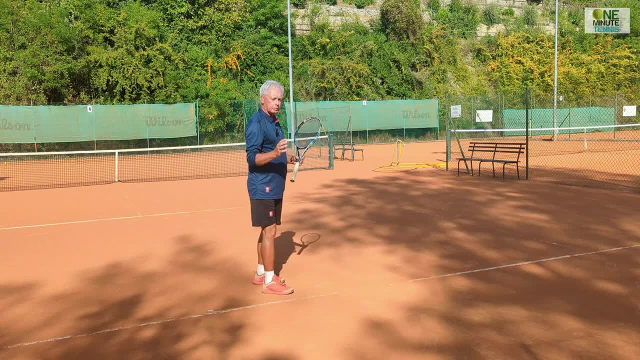 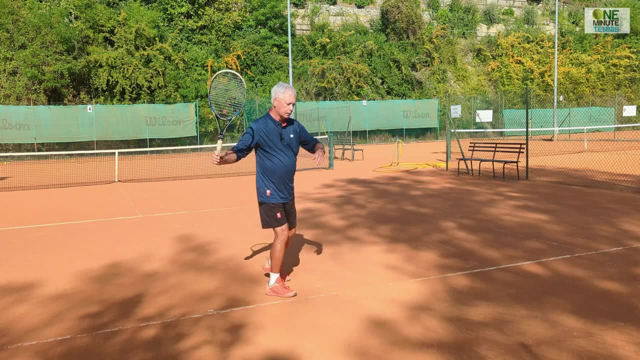 through the ball. If you look in this direction, the difference between me setting up normally and setting up inside the shelf- Let's do the high ball to begin. So I set up normally, swing from down here, And this is an ineffective stroke And I'm now in the weak area Up here. my arm is very weak, So I 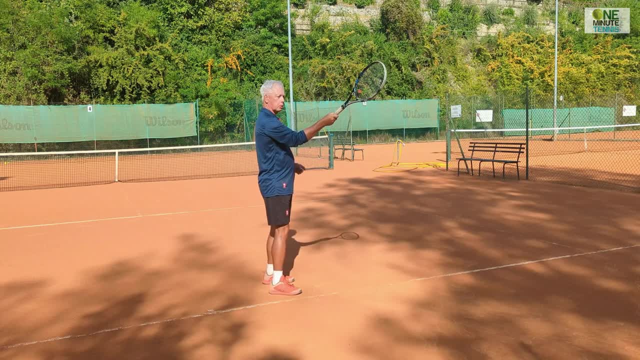 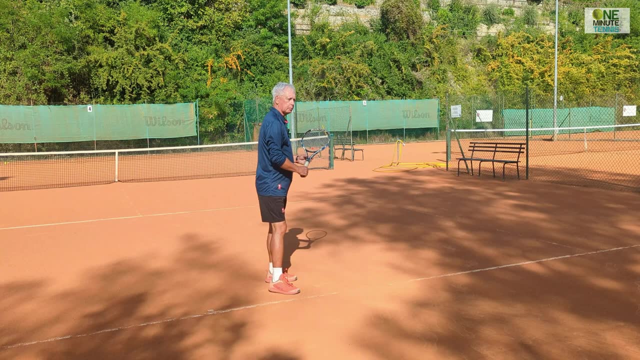 have a combination of problems: A lack of physical strength for adjustment and controlling and accelerating the racket And a very awkward swing across the line of the ball. But now I set up in the shelf, So I'm in the shelf and I swing through the ball. I'm in the shelf and I swing through the. 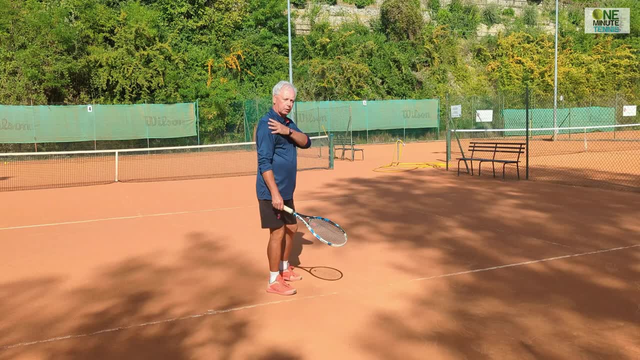 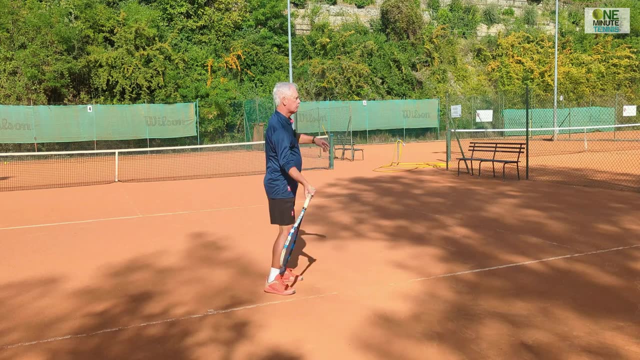 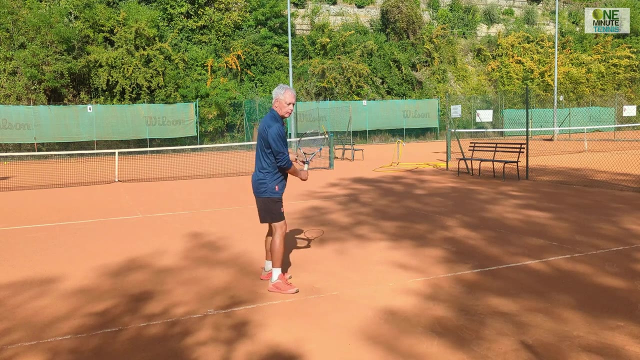 ball And from this position, I'm using my deltoids, my shoulders, rather than my biceps, And my shoulders are still strong at this height, But my bicep is weak at this height, Now going to a more preferable height, So I have my normal take back, Oh, and I'm in the shelf. In the shelf and swing through. 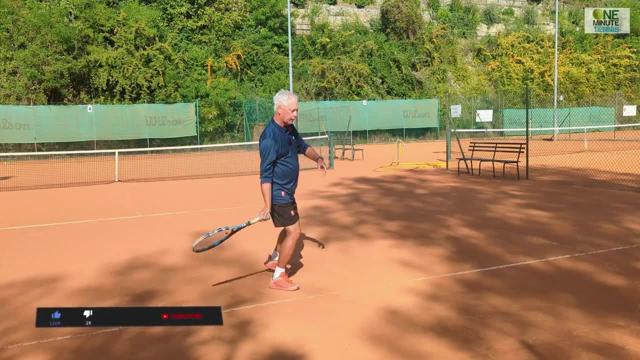 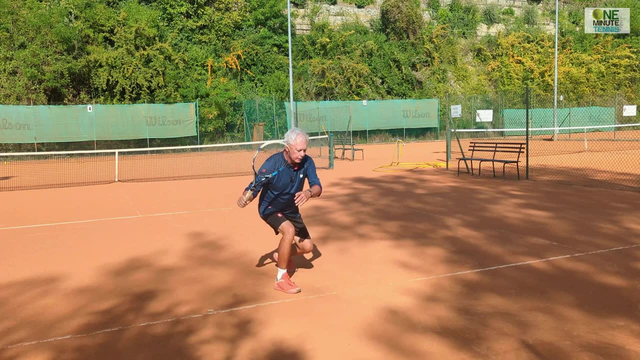 the ball. Now for the low ball. Let's have a look at the normal take back. My body is too upright. I have this awkward position here and a lot to do with the hand, But now I get in the shelf. and to get in the shelf, to get.